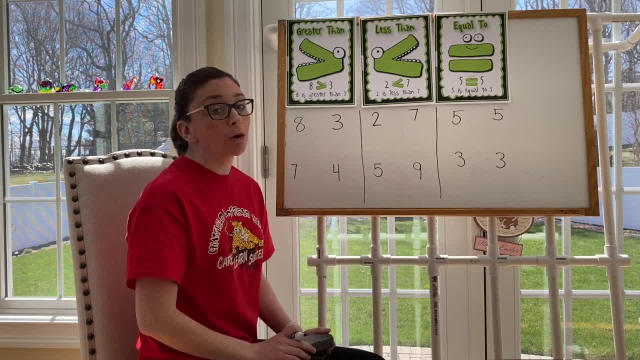 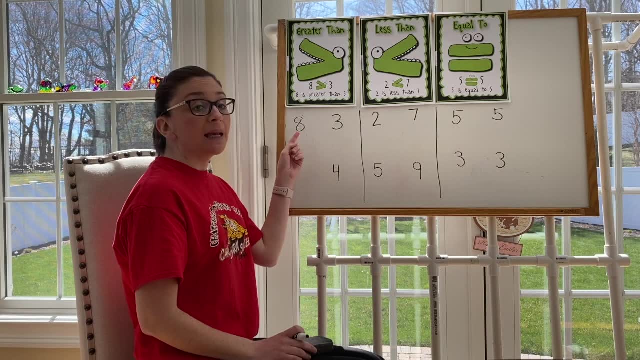 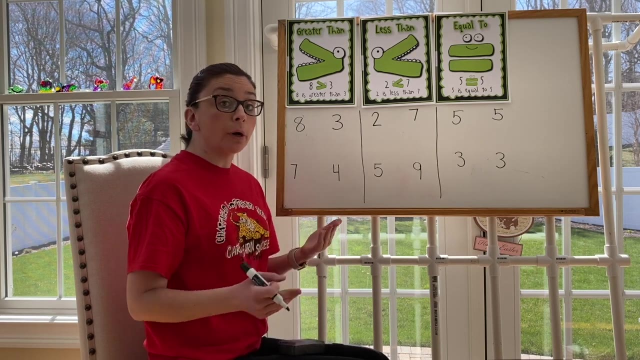 Hi, boys and girls. Today I'm going to teach you about greater than, less than and equal. So let's start with greater. I have two numbers right here, eight and three. I need to find which number is greater. Well, the word greater means more. So which number has more? If you're not sure, you 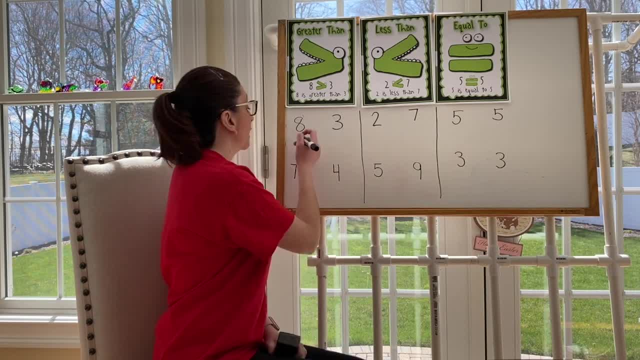 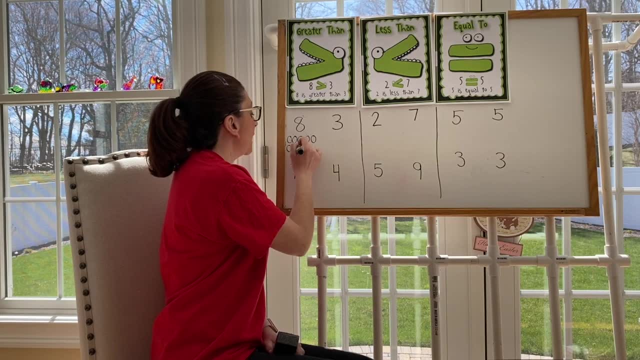 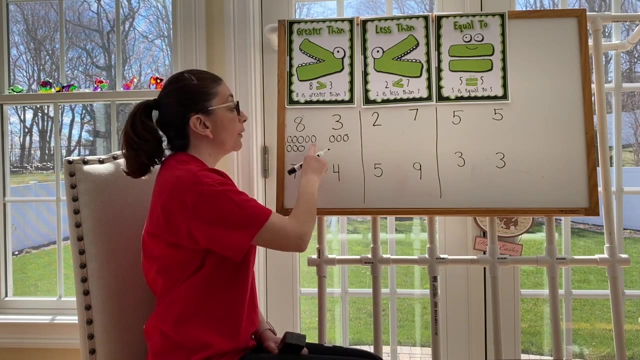 can always draw circles underneath each number. Let's start with eight. One, two, three, four, five, six, seven, eight. Now let's look at three. One, two, three. Which number is greater or has more? The number eight. 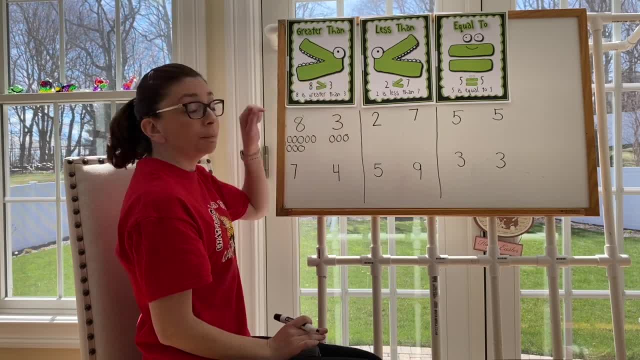 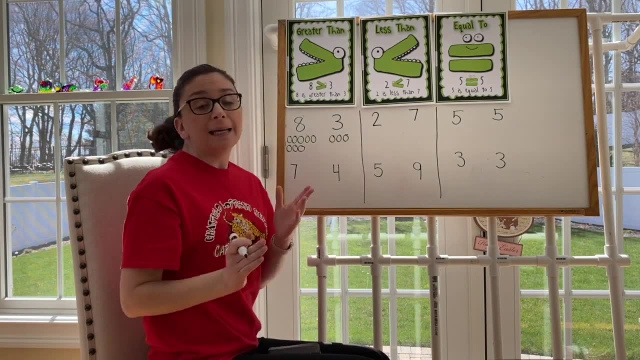 Now, if you look up here, you will see a symbol. It kind of looks like an alligator mouth Protect. Let's pretend that this arrow is an alligator mouth. An alligator is always hungry. Does he want to eat a small? 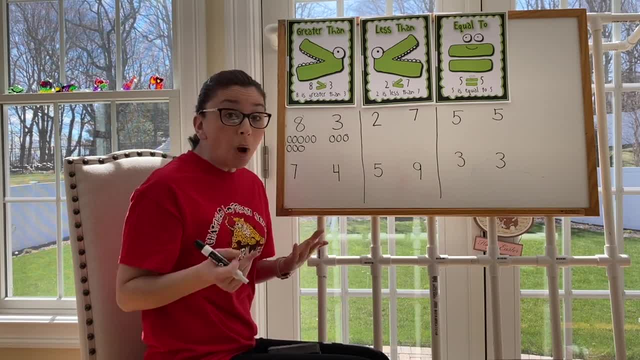 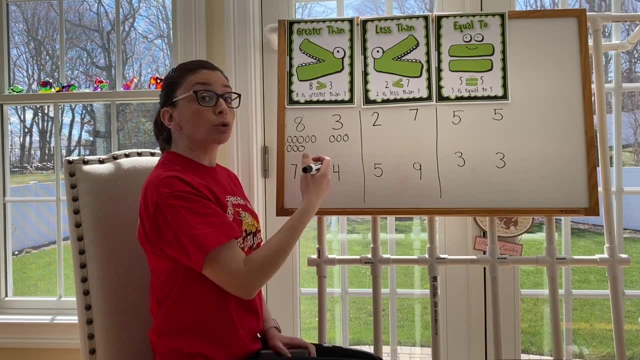 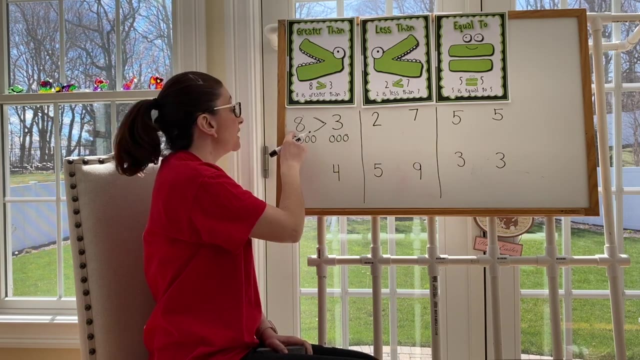 amount, or the biggest amount He wants to eat, the biggest amount. So when I draw my arrow, if I'm saying a number is greater, I need to make sure that the biggest part of my arrow faces the bigger number. the greater number I'm going. 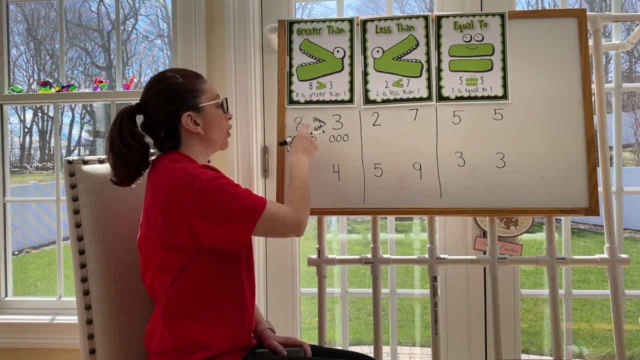 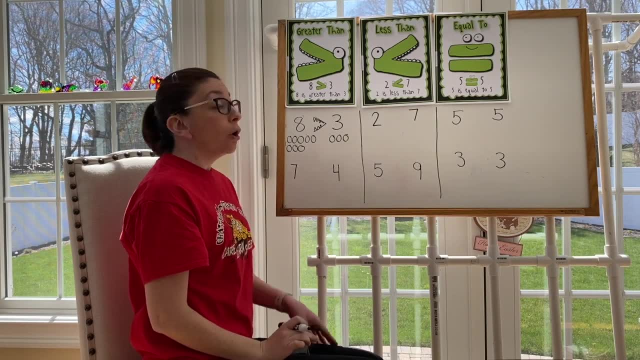 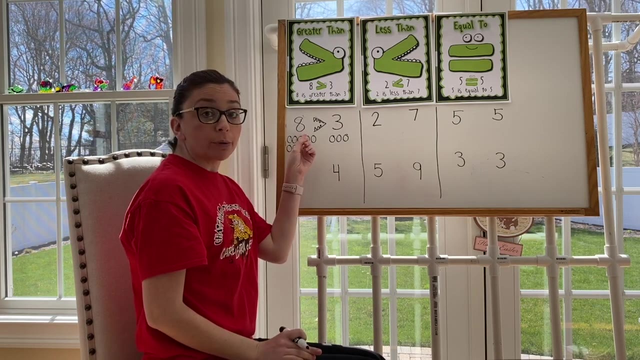 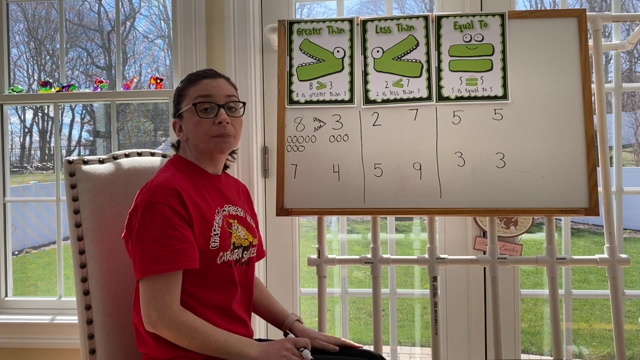 to pretend that my alligator has teeth and he's going to eat that number eight. When we're talking about greater, then we look at the arrow and the open end always goes toward the bigger number, the greater number. Let's look at another example: Seven and four: Which number is greater? 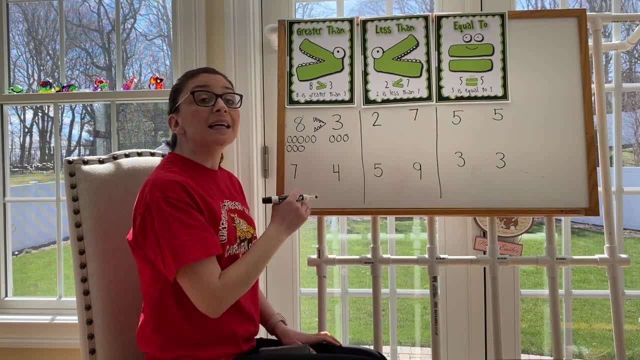 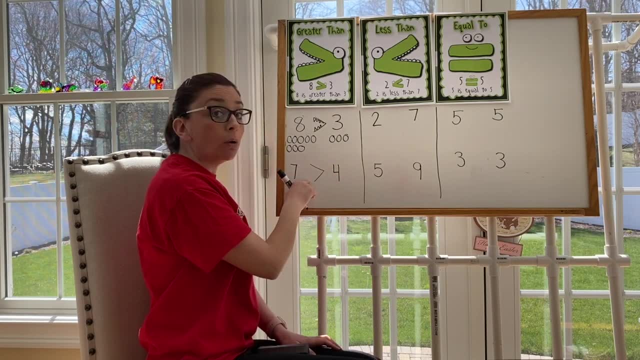 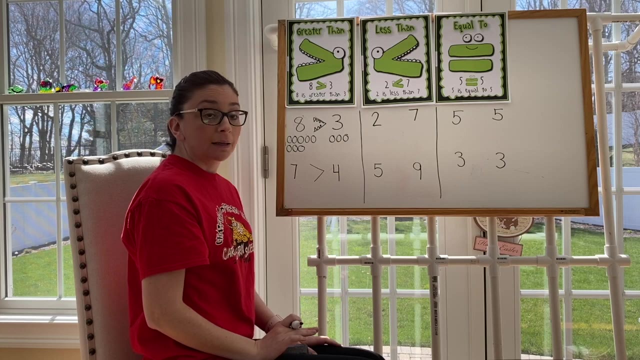 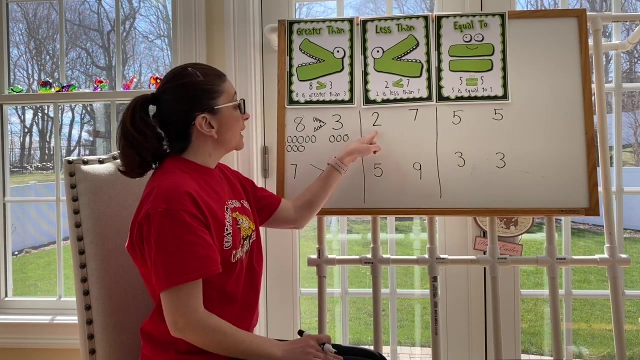 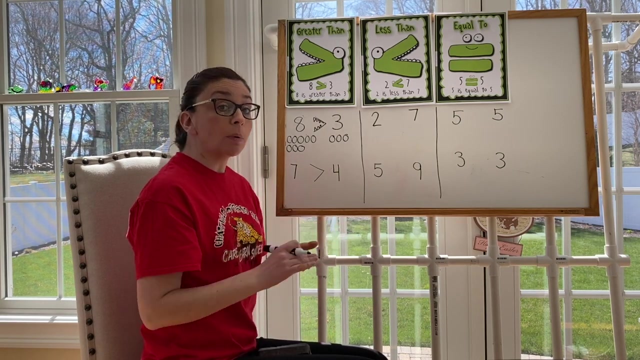 Seven is greater. Seven is the greater number. It has more. So when I draw my arrow, I need to make sure the big end of my arrow, or my pretend alligator mouth, is facing the bigger number. Let's look at less than Less, than means smaller. So let's look at these two numbers, two and seven. If I don't know how to tell which number is greater, I need to make sure that the big end of my arrow, or my pretend alligator mouth, is facing the bigger number. 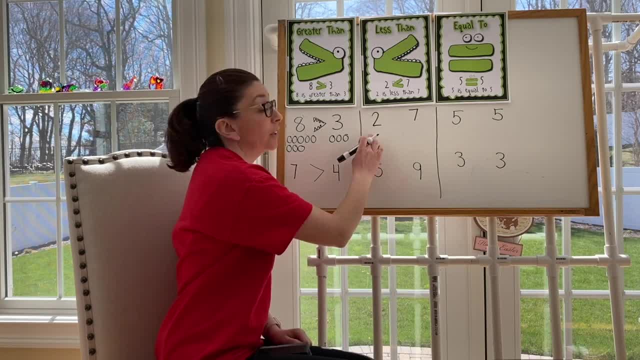 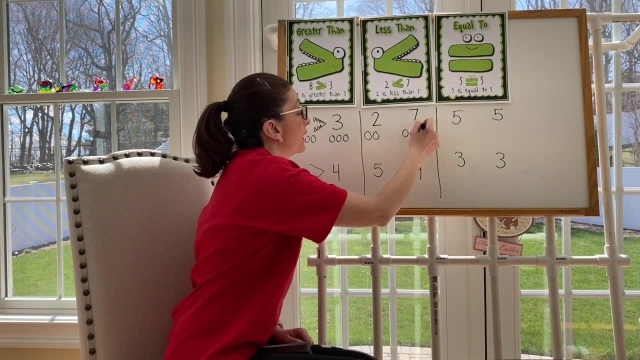 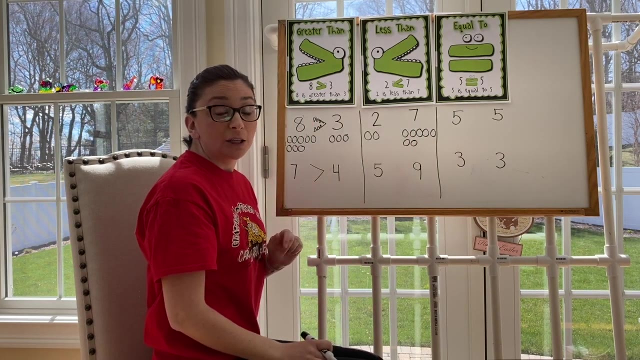 If I know I can always draw my circles Two, one, two, Two, one, two and seven. One, two, three, four, five, six, seven. Which number is less? Two is less. When I'm talking about a number that is less and I'm using my arrows, I need to make sure the small part of my arrow faces the smaller number and I see two circles with pink eyes. I'll want to filling each mark with the ranks and three in between Two circles, But here's one. Now I'm going to call each number and let me draw the numbers fourth on the left and fifth on the right. Let me go around again and even out the position of the questions. If I can always draw my circles- two, one, two and seven. One, two, three, four, five, six, seven- Which number matters�? Officer, teacher is always. 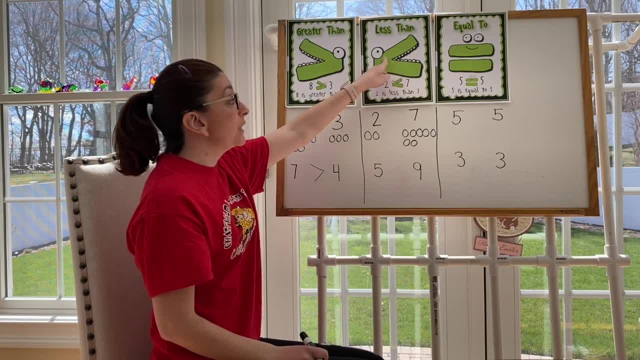 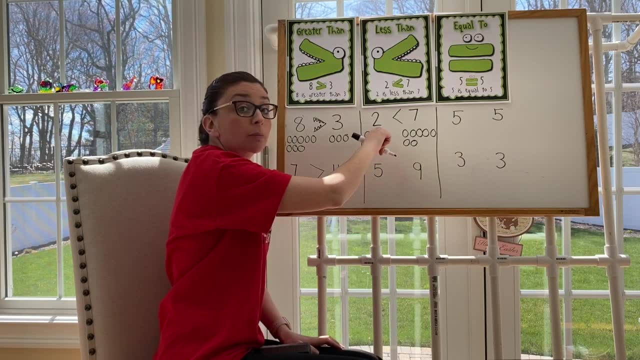 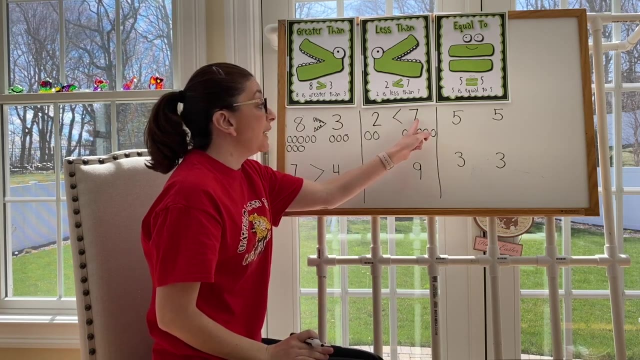 When I'm talking about a number that is less and I'm using my arrows, I need to make sure the small part of my arrow faces the smaller number, the number that is less. If you look at the mouth of my arrow, it's still eating or facing the bigger number. Let's look at 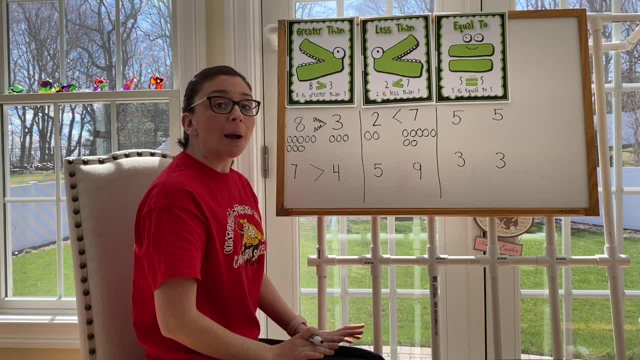 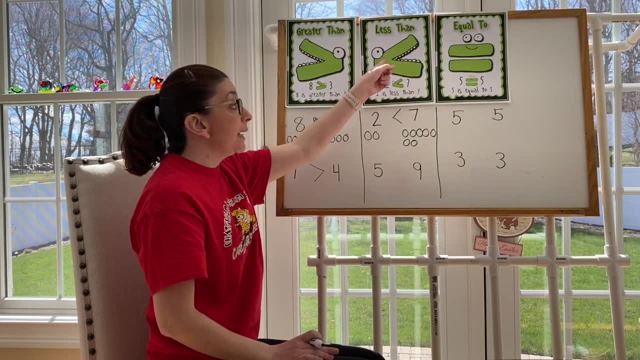 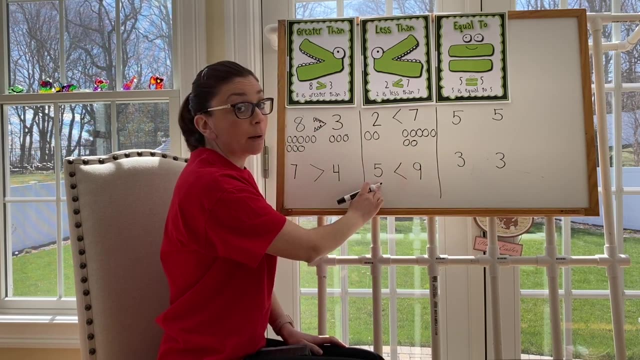 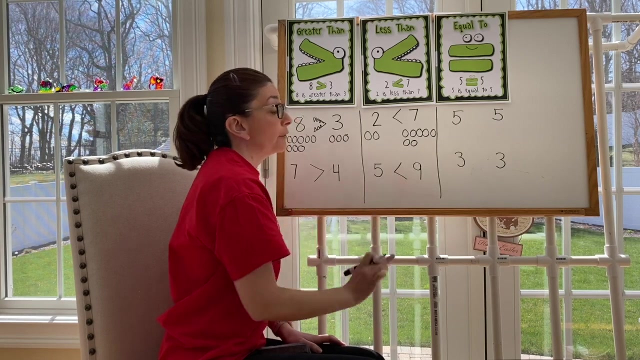 the numbers five and nine. Which number is less? Five is less. So I look at my arrow and the small part. the point of my arrow faces the smaller number, the number that is less, and the bigger part, the open part, faces the number that is. 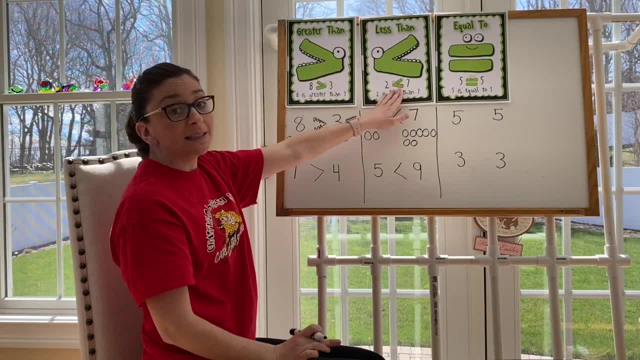 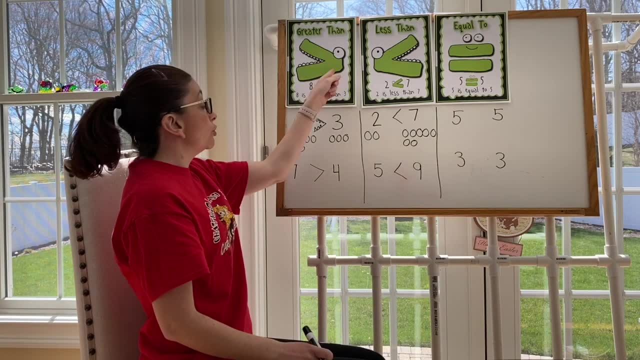 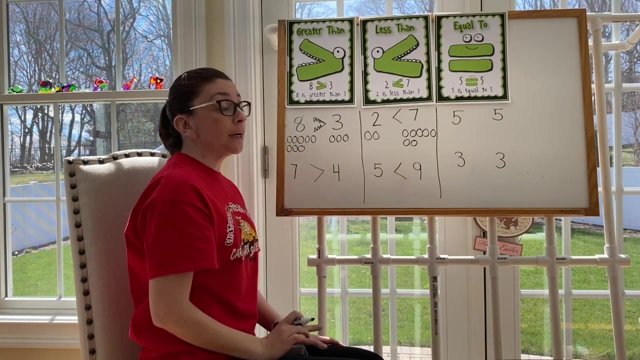 more. Let's review greater than and less than before we move on to the next example. So greater means more. When you use your arrow, you want the wide end of your arrow to face that bigger number. Eight is greater than three. Seven is. 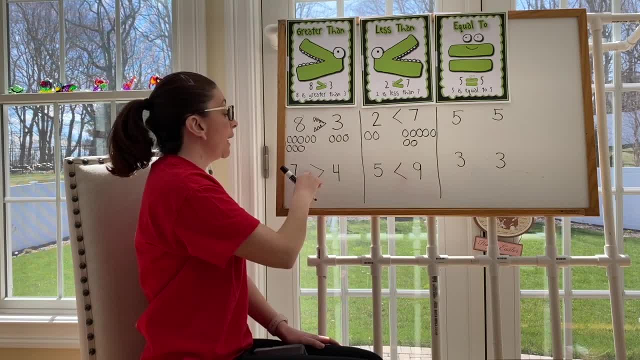 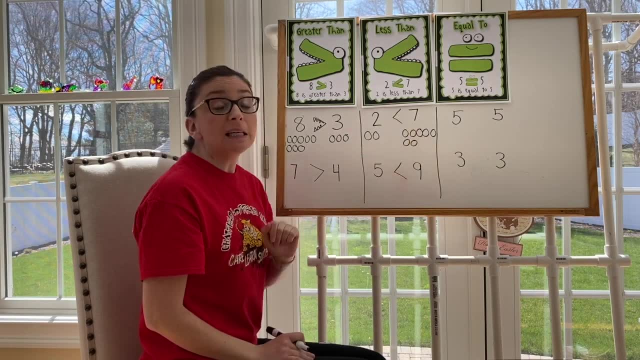 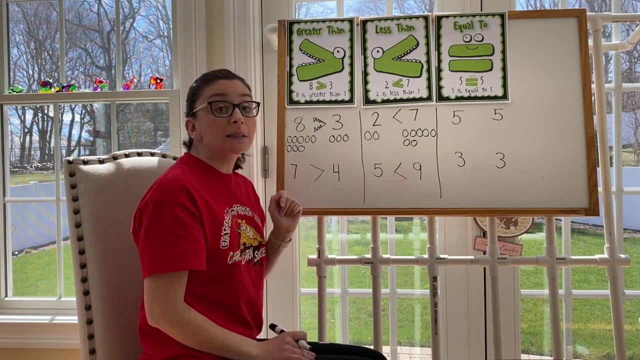 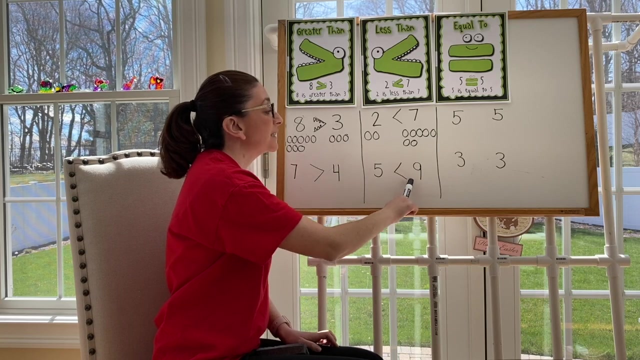 greater than four. The bigger part of my arrow faces the bigger number. When we talk about less than that, pointy part of the arrow faces the smaller number. So the smallest part of the arrow faces the smaller number. Two is less than seven. Five is less than nine. Now let's talk. 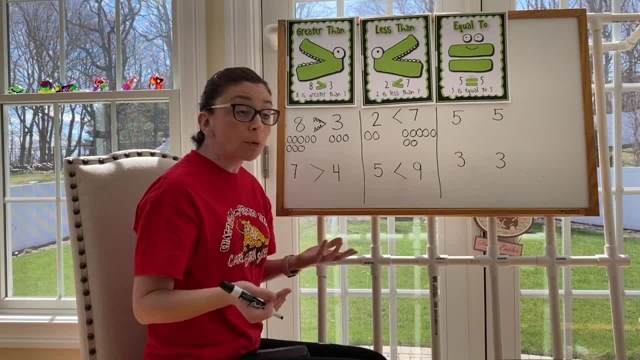 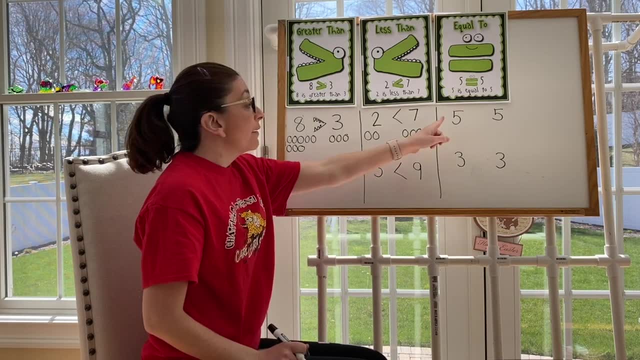 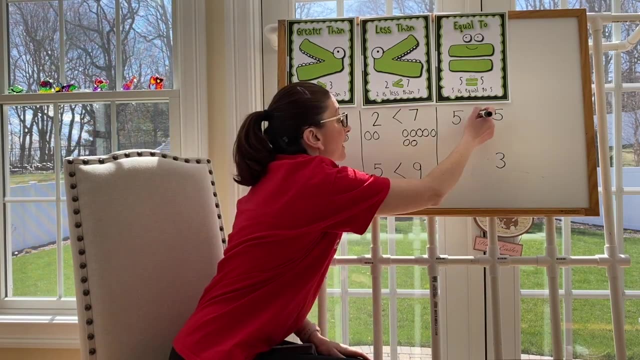 about equal and we're all familiar with the word equal. Equal means that both numbers are exactly the same. Five and five. are they the same? They are, So we would say that they are equal. Three and three are they the same? 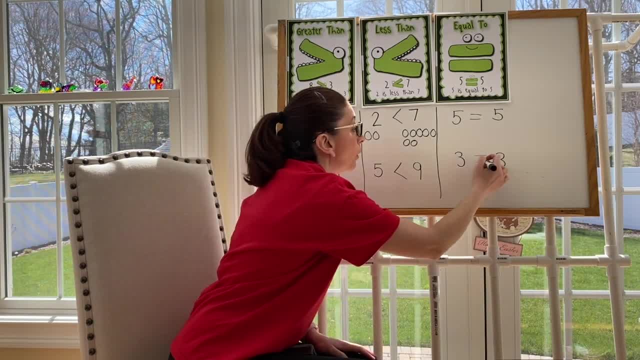 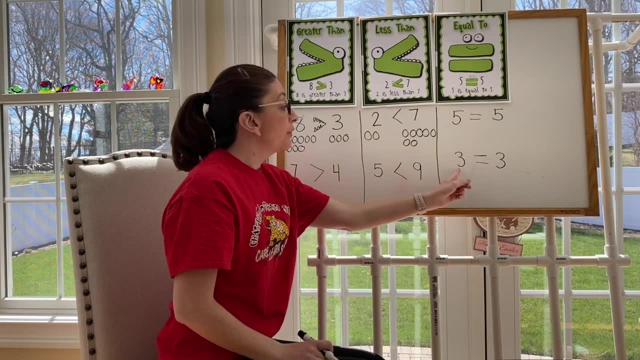 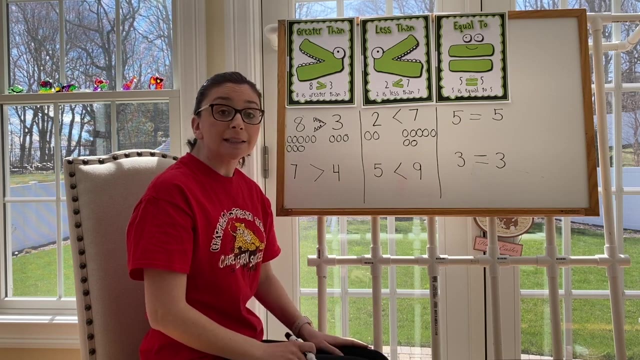 They are. So we would say they are equal And you would read your problem as: five is equal to five, Three is equal to three. I hope this helps boys and girls. You have some practice work to do If you have any questions. 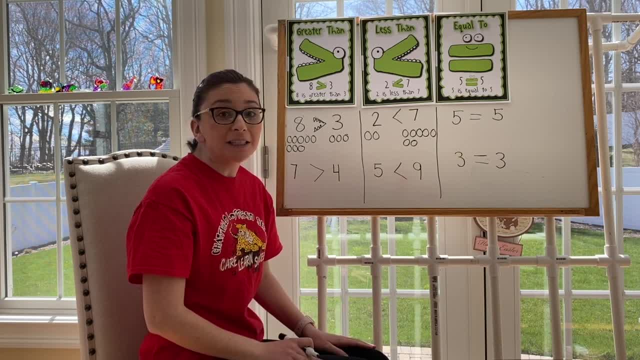 feel free to have mom and dad email your teachers. Have a good day. 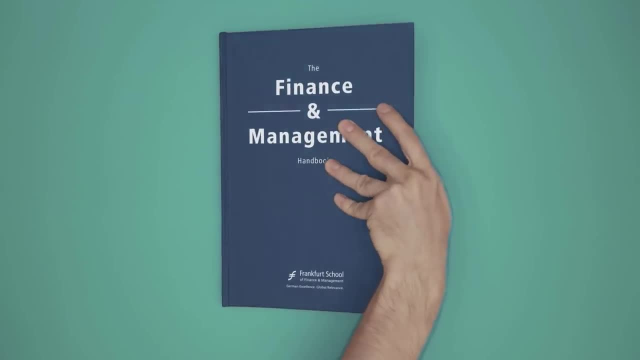 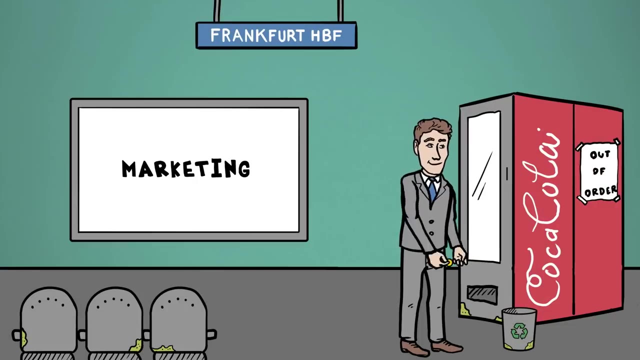 Okay, let's do this Today. I'm going to teach you what consumer behavior is. First of all, it is defined as the area of research within the field of marketing that focuses on how consumers acquire, use and dispose of goods, services, time and ideas. 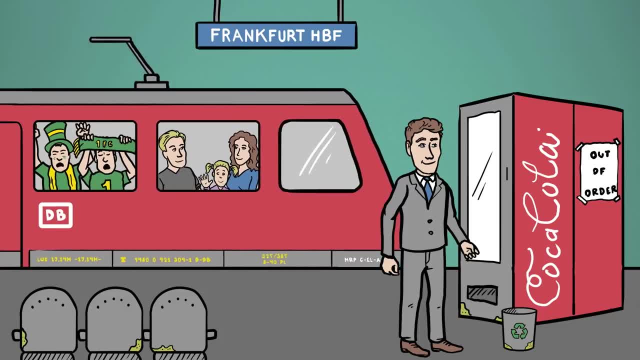 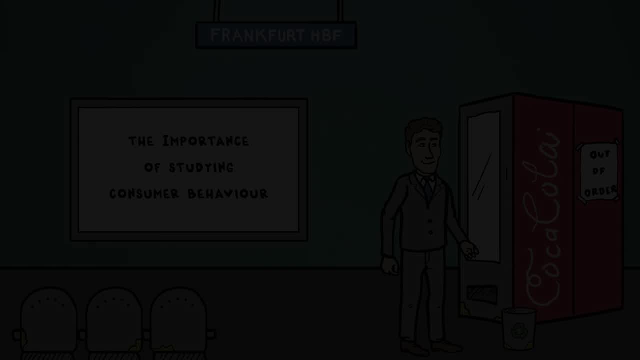 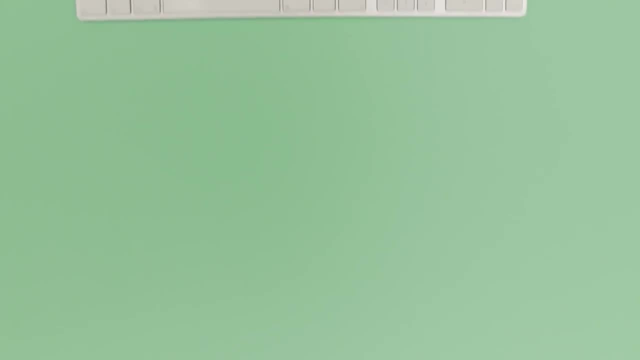 Consumers can be individuals, families or other groups such as teams and companies. Let's try to understand the importance of studying consumer behavior. Suppose you need a new phone. How would you go about satisfying this need? Where would you turn to for information? 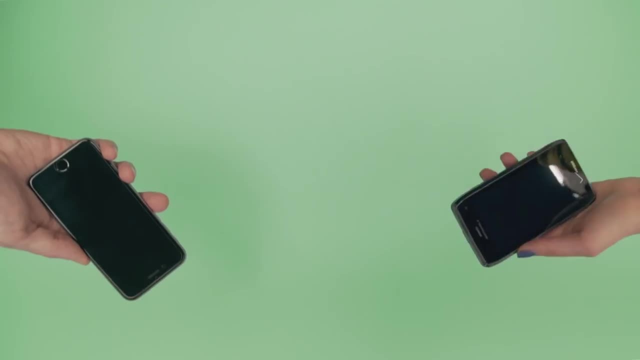 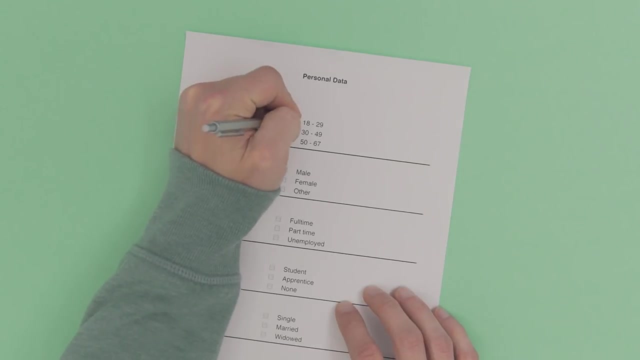 How would you set your budget? Where would you buy the phone? These are just some decisions consumers face on a regular basis. Interestingly, each consumer will answer these questions differently based on their backgrounds and some psychological factors. For a company that makes phones, 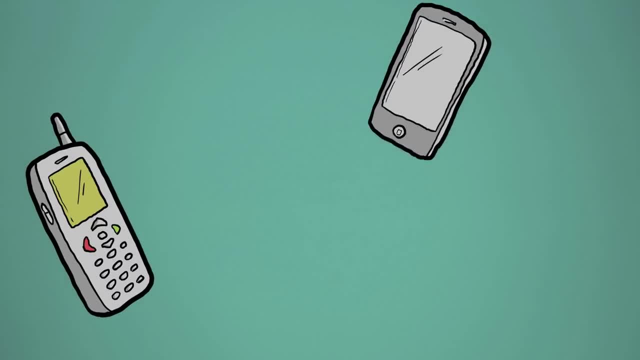 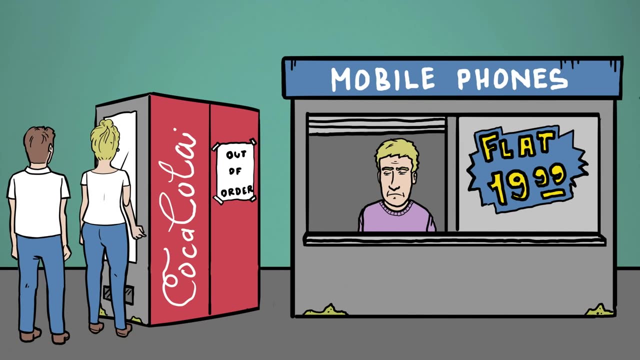 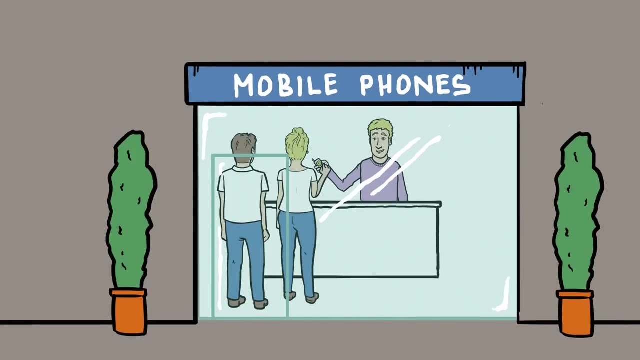 the answers to these questions will help them know the types of phones to design, the price consumers are willing to pay and where they should sell their phones. It is very important to understand how consumers make decisions, because the best way to create and keep customers is to understand what motivates their consumption decisions. 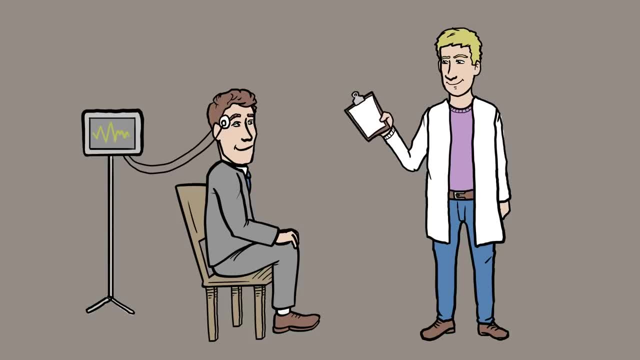 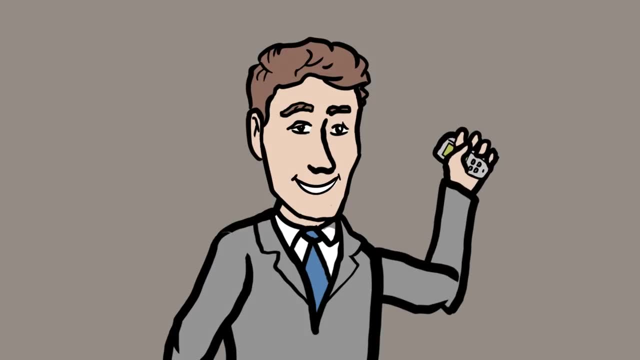 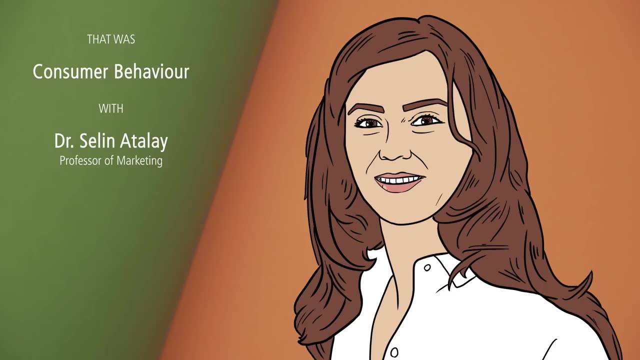 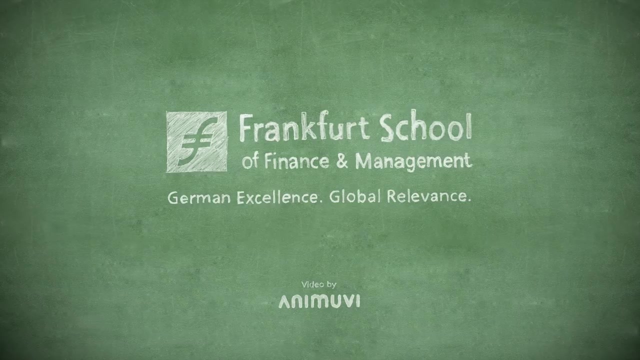 and anticipate their consumption needs. Only this way companies can design products, services and offers that will make their customers happy. How would you explain when you might affect your consumers? Please leave your survey informed. I would like to tell a few things about your się ting. 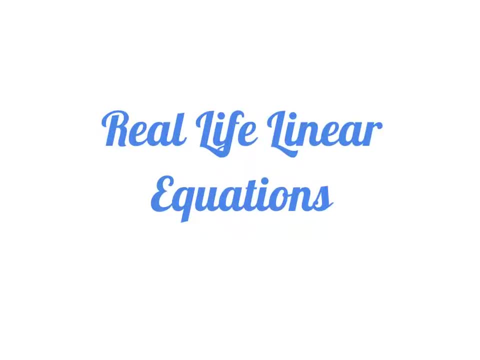 Hi everybody. Today we are going to be creating real-life linear equations. So today, since we're doing real-life linear equations, we are essentially going to be working with some word problems, And any time that we're going to do word problems, I'm